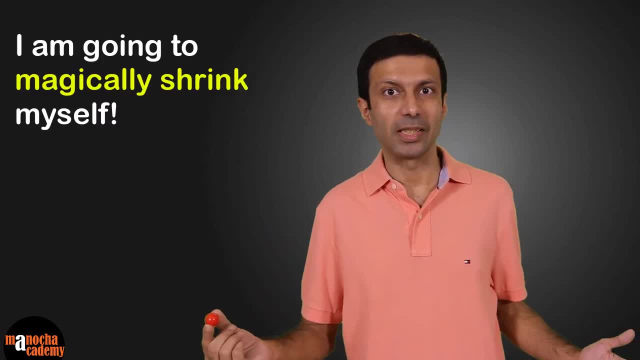 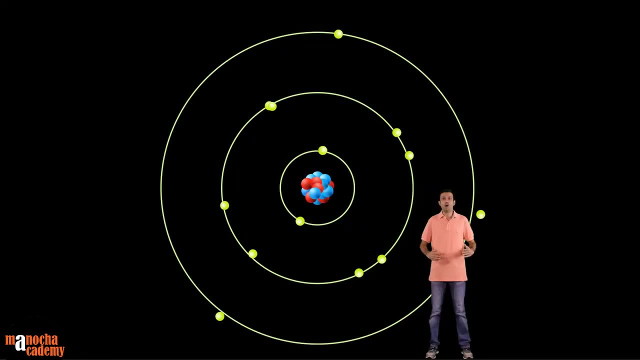 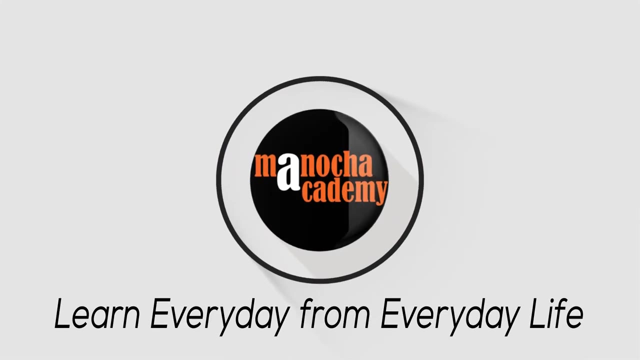 In this video I'm going to magically shrink myself like a trillion times smaller And I'm going to enter this atom. Let's explore what's in this tiny particle. Hi friends, I'm sure you've heard the word atom in chemistry. 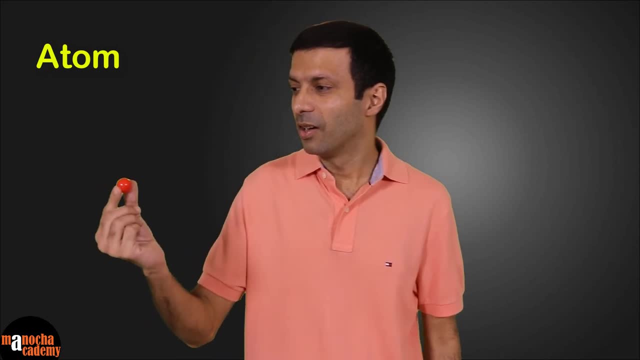 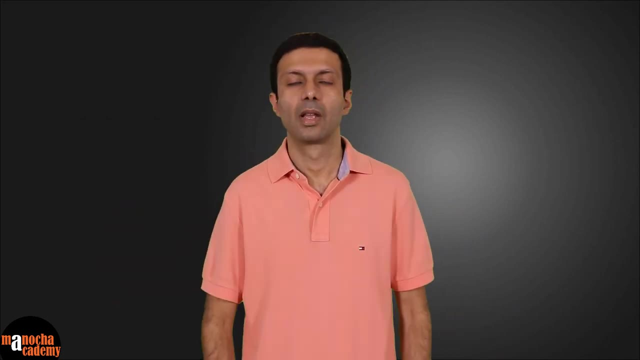 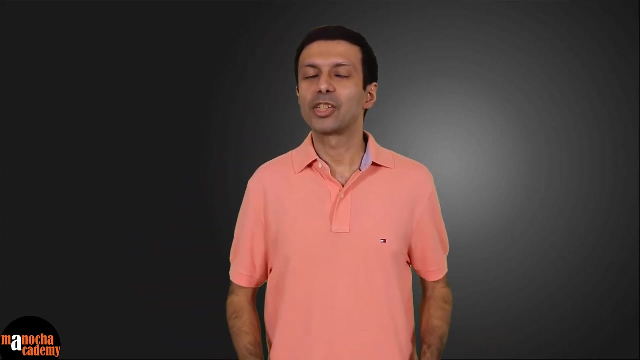 It's a very tiny particle. Here I have a model of an atom. The real atom is so tiny that we can't even see it. Before I become really tiny and we go on a journey inside the atom, let me ask you: what does the word atom mean? 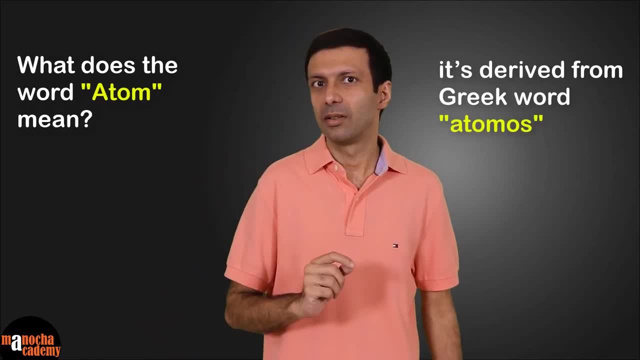 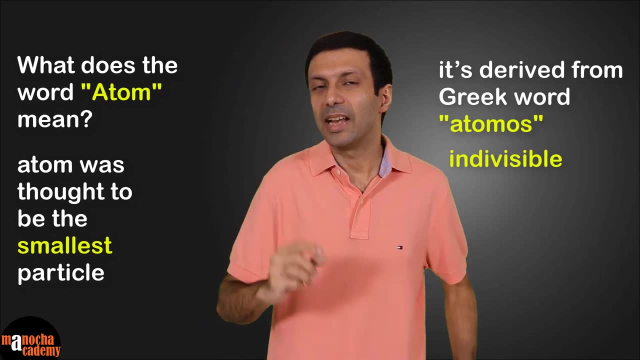 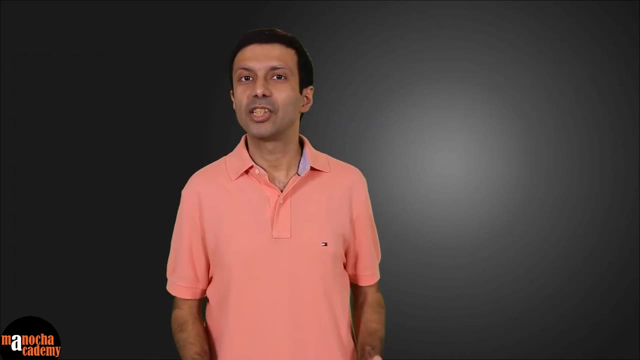 It's derived from the Greek word atomos, meaning indivisible, Because they thought that the atom is the smallest particle and it cannot be divided further. But now we know that's not true. Scientists such as Thomson, Rutherford and Chadwick. they discovered subatomic particles. 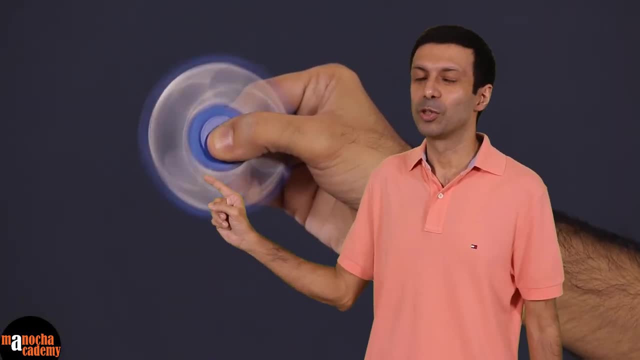 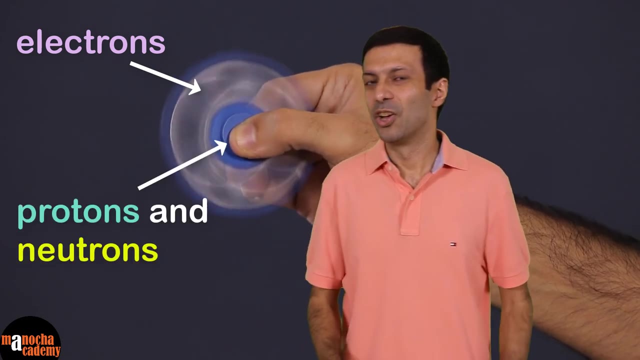 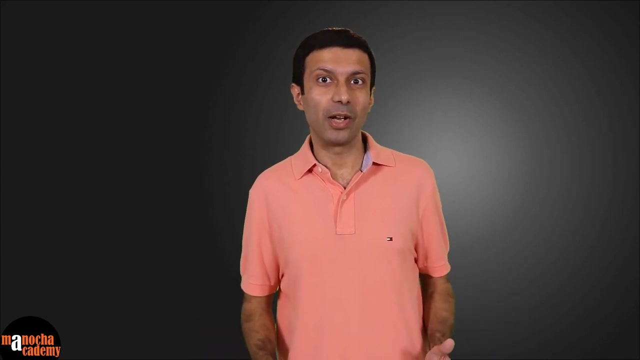 I have a video on Thomson's and Rutherford's model of an atom. In this video, I compare the structure of an atom to a fidget spinner, So do check it out. Alright, friends, wish me luck, Because I'm going to shrink myself. 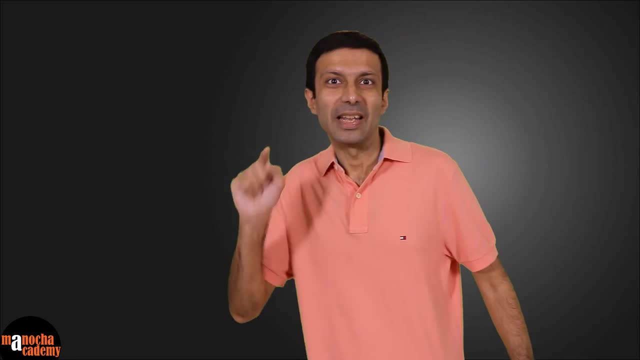 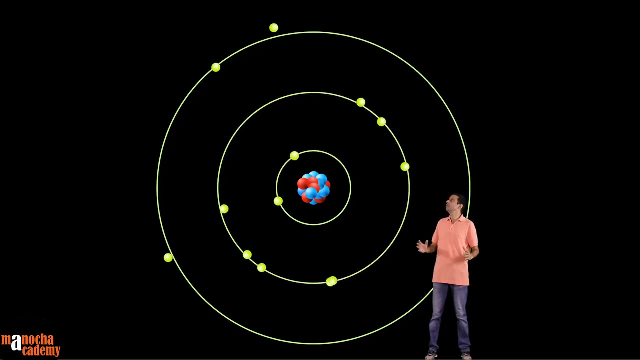 Like a trillion times smaller And we are going to go inside the atom. Alright, we are inside the atom. now The atom looks mostly empty, hollow. Wait a minute. I can see some tiny particles spinning around here. There's also something in the center. 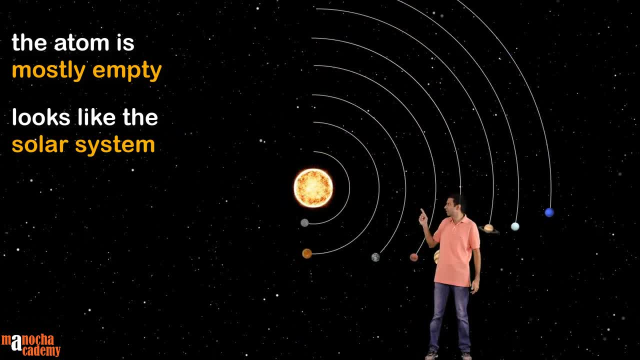 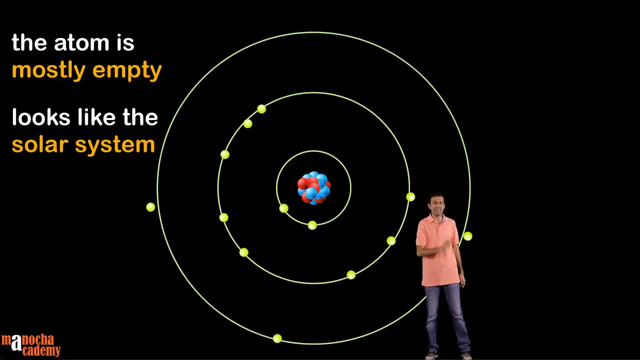 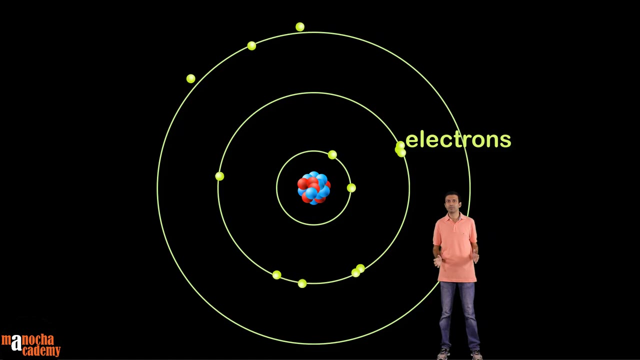 This looks like a model of the solar system, With the sun in the center and the planets spinning, Spinning around it. Now let's look at each part in detail. The tiny particles spinning around the center are called electrons. These are negatively charged particles and they have a very small mass. 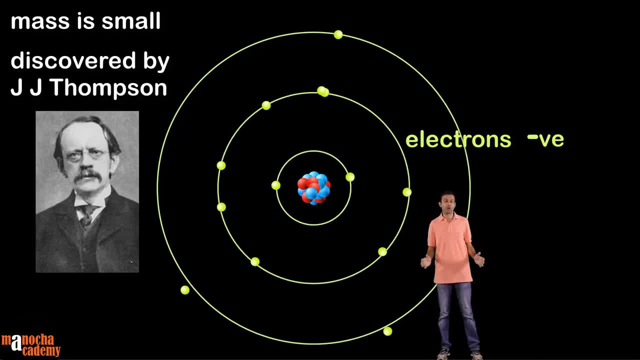 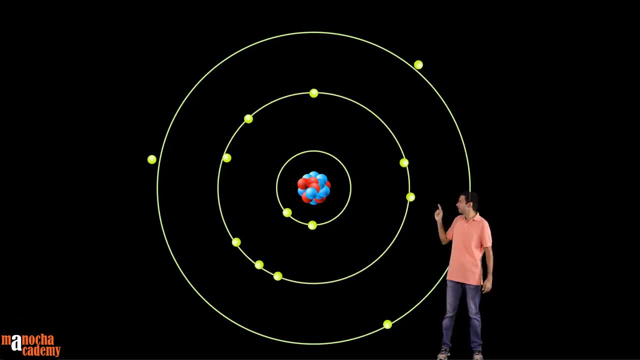 The electrons were discovered by J J Thomson using the cathode ray tube experiment. Can you see that there's something in the center of the atom? Can you see that there's something in the center of the atom? Can you see that there's something in the center of the atom? 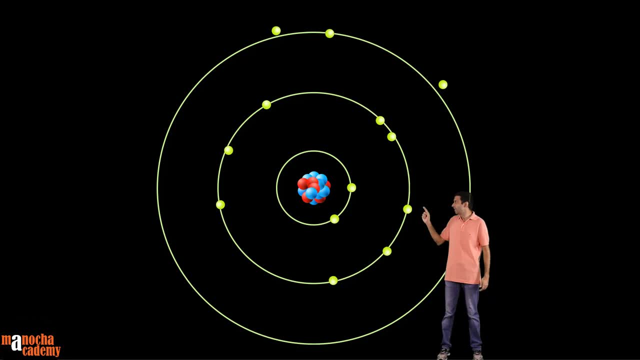 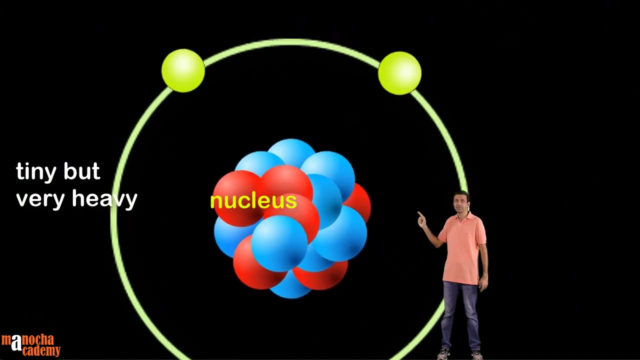 Remember Rutherford's model of the atom. Remember Rutherford's model of the atom. He called the center, the nucleus. The nucleus is very tiny but holds almost the entire mass of the atom. So let's zoom into the nucleus and let's see what's inside it. 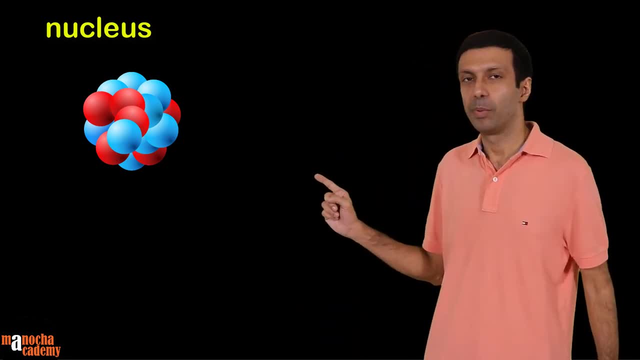 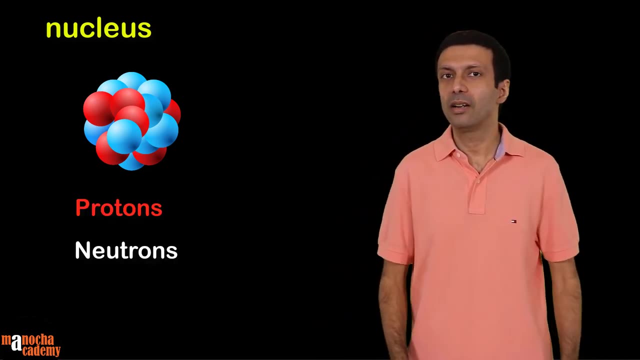 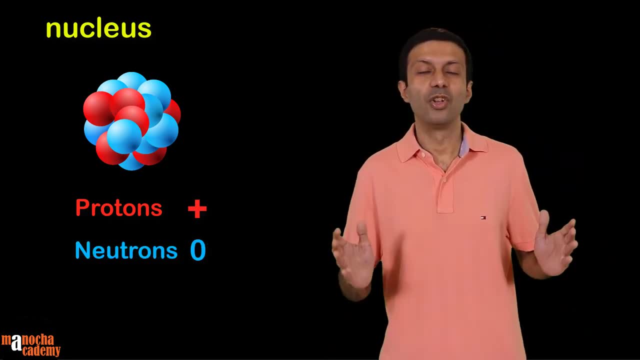 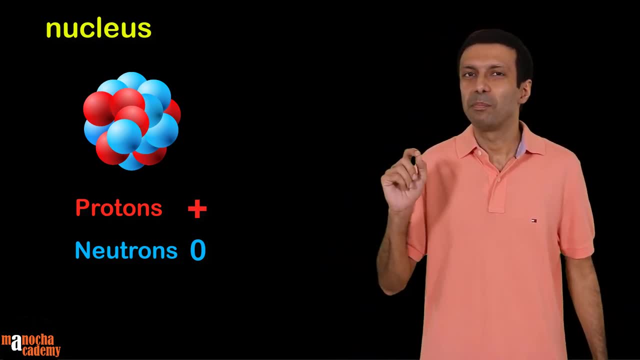 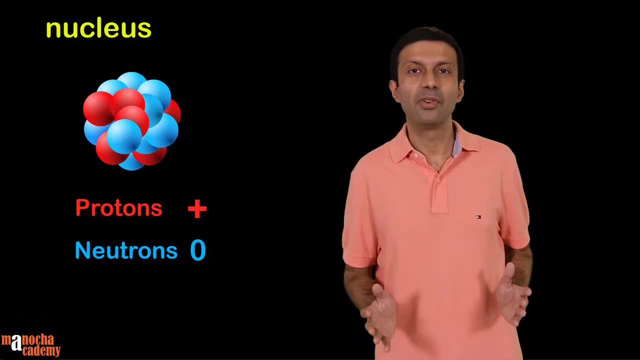 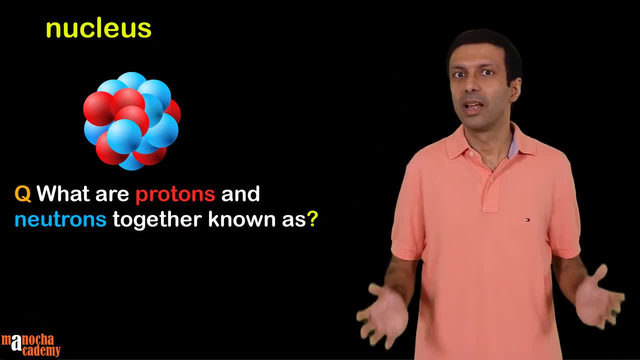 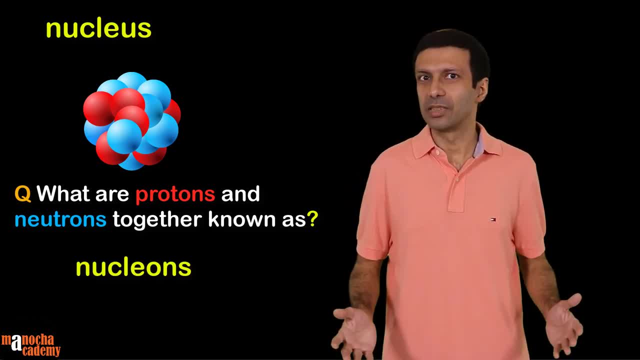 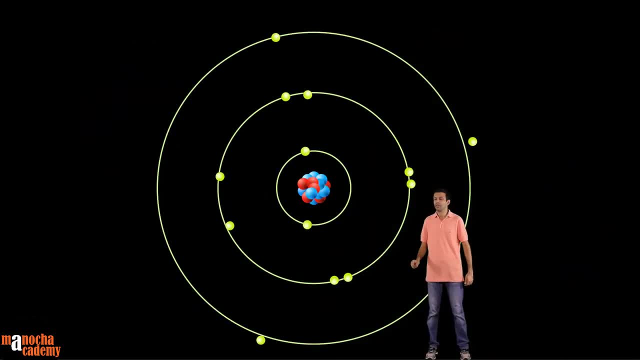 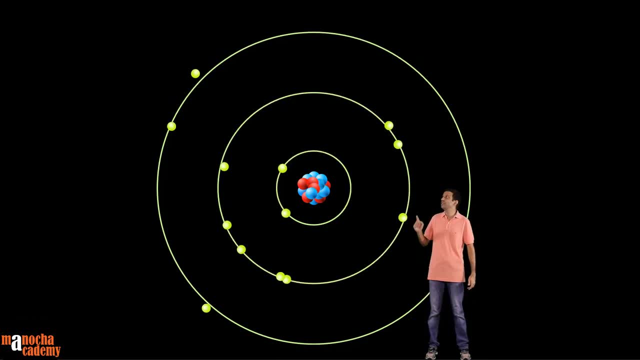 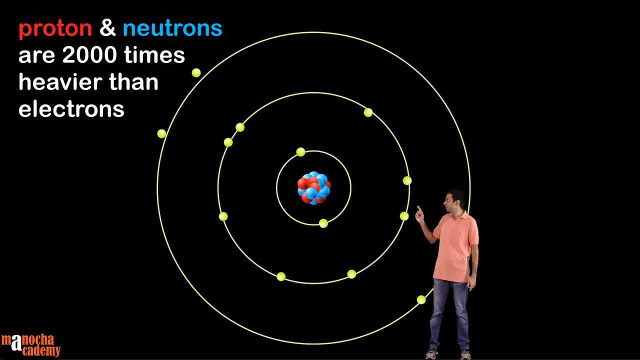 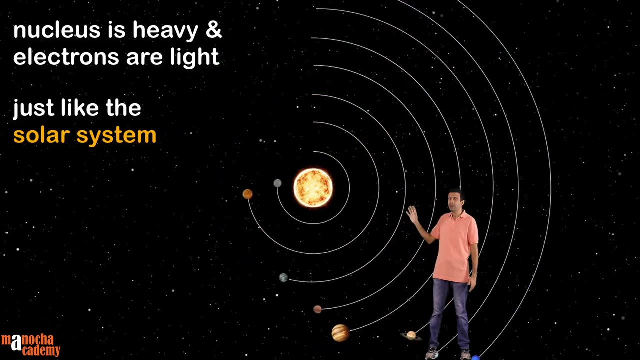 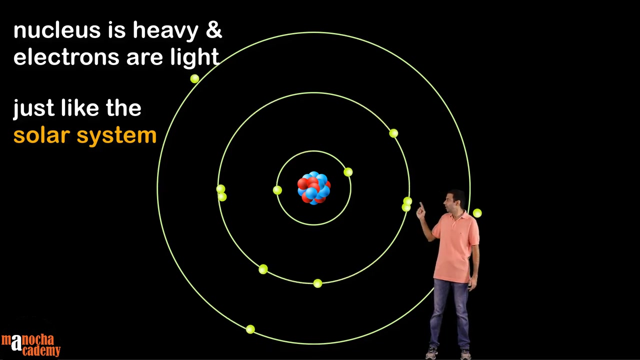 So almost the entire mass of the atom is sitting in the nucleus. here The atom has this very heavy nucleus with the light electrons spinning around it. It's just like the solar system, with a very heavy sun and light planets spinning around it. Now do you know what's in the space between the nucleus and the electrons? 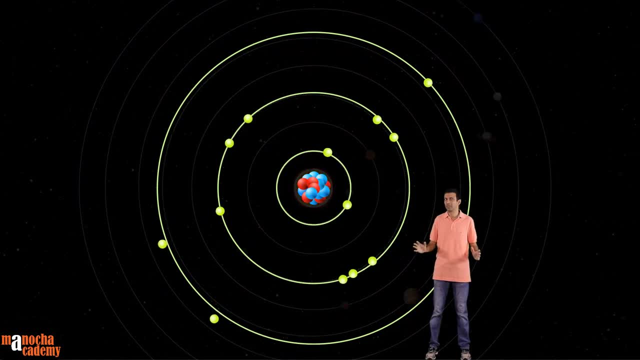 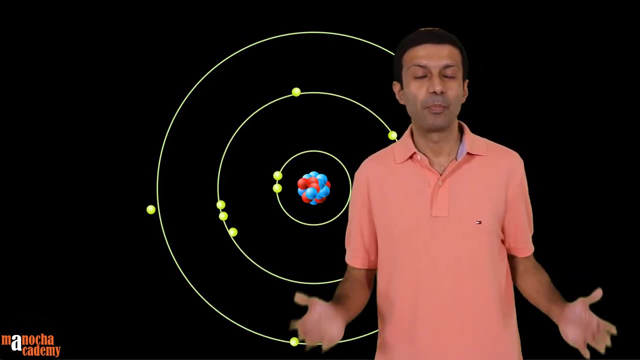 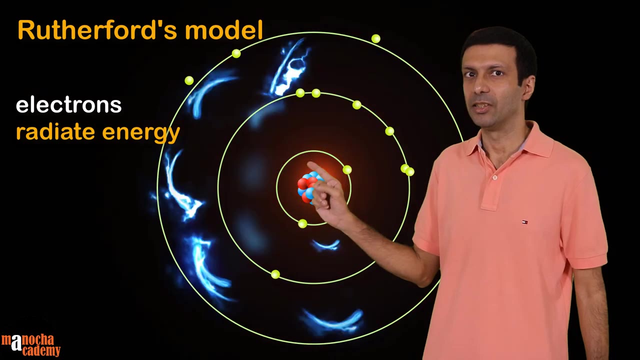 Again, it's just like the solar system. This is just empty space, It's just vacuum. But there was a problem with Rutherford's model of an atom. The electrons revolving around it would radiate energy. This means the electrons would lose energy and finally fall into the nucleus. 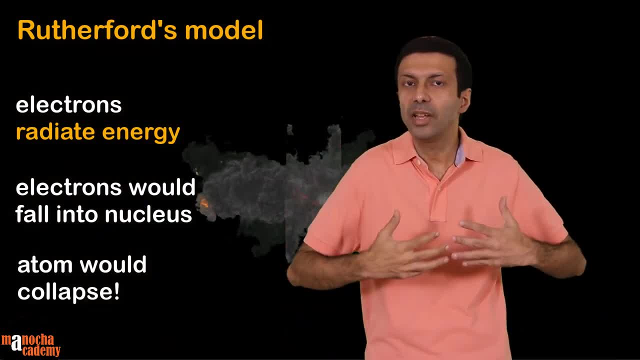 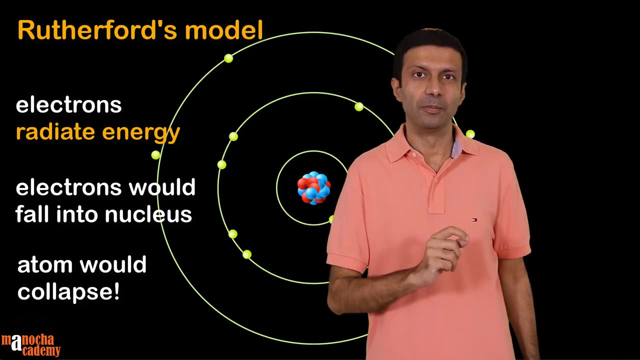 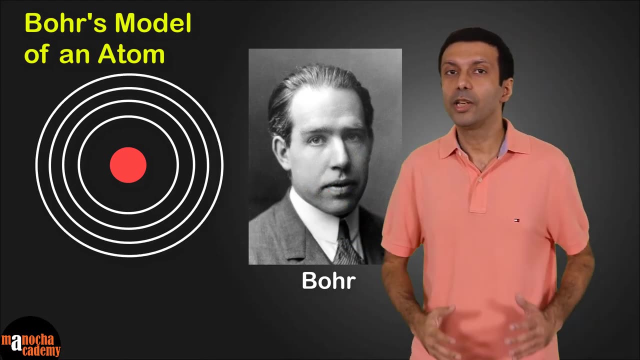 So the atom would collapse, Then everything around us should collapse. But we know that's not true. The atom is stable, So Bohr proposed a new model of an atom to correct this. According to Bohr's model of an atom, the electrons can revolve around the nucleus. 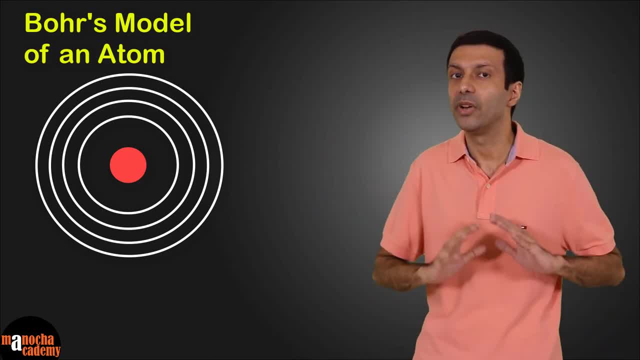 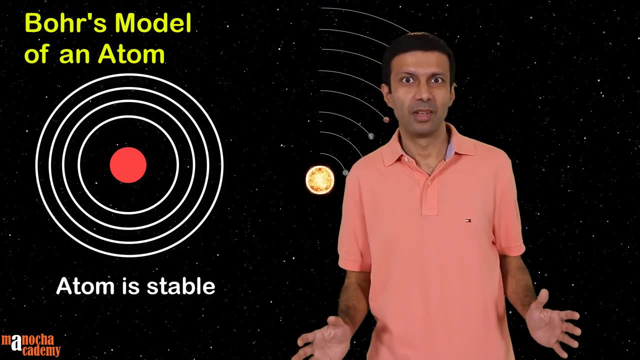 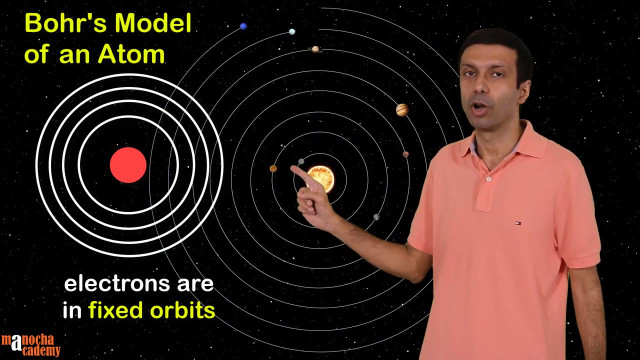 The electrons can revolve only in certain orbits where they do not radiate energy. So the atom is stable. It's just like the solar system, where the planets revolve around the sun in fixed orbits. So let's take a look at Bohr's model of the atom. 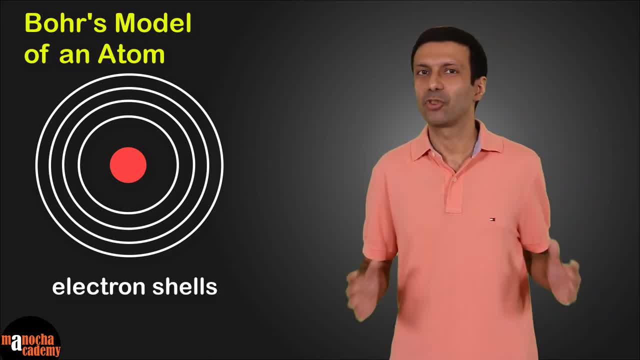 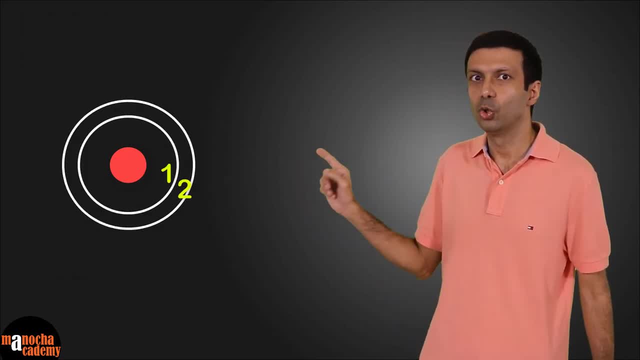 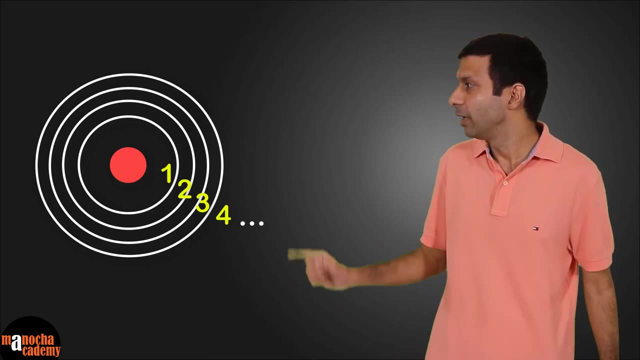 The fixed orbits in an atom are known as electron shells. The shells are numbered starting from the innermost shell, So it's 1,, 2, 3, 4 and so on, Or they are labelled using letters, starting with the letter K. 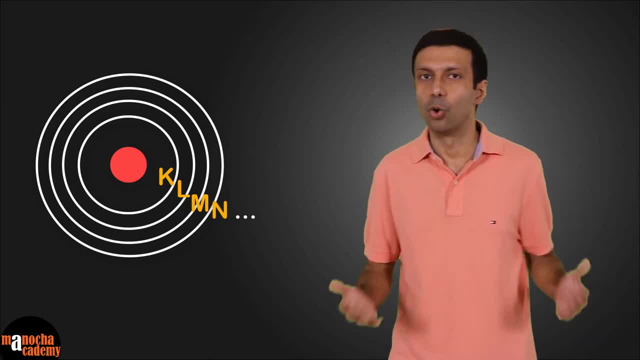 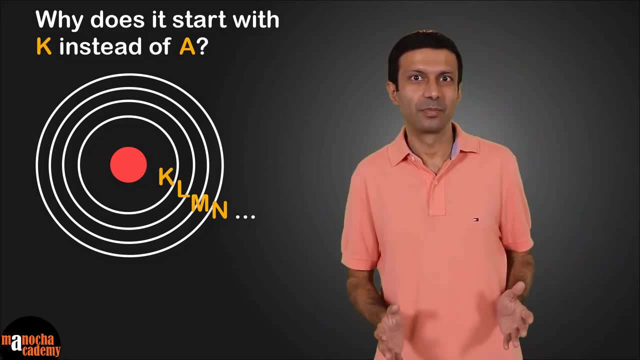 So it's K, L, M, N and so on. Now you may be wondering: why do they start with the letter K? Why is it not A? Well, there's an interesting story behind this. I would encourage you to find it yourself. 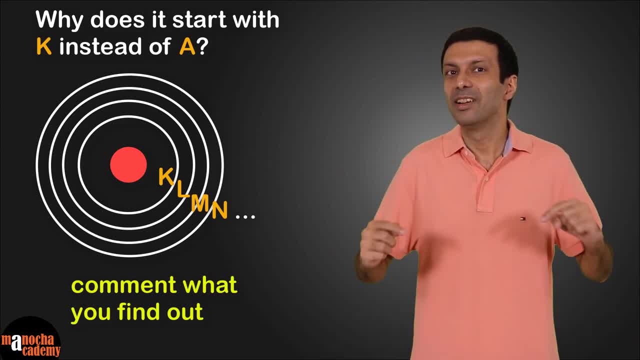 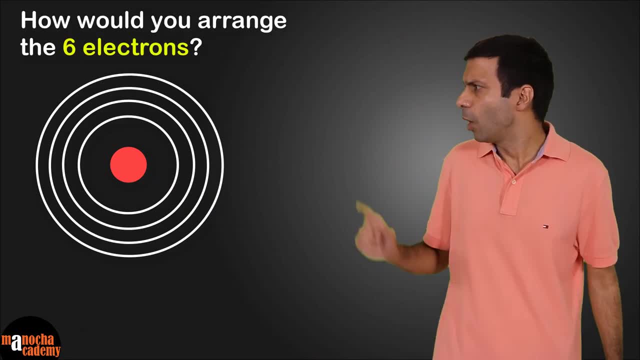 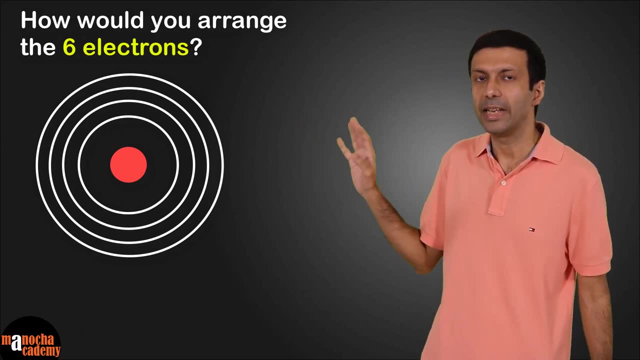 And do let me know what you found By putting it in the comments below. Now, let's say, an atom has 6 electrons in it, So how would you arrange the electrons in these different shells? Can we just put them randomly in any shell? 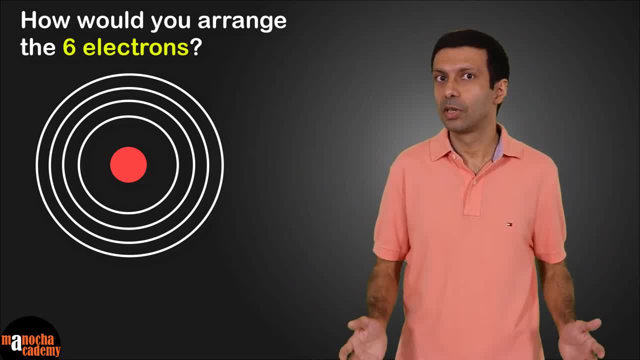 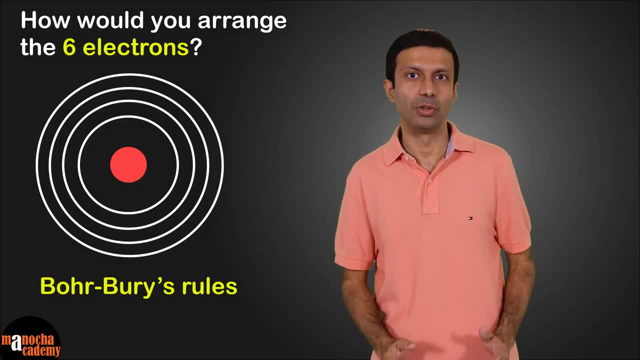 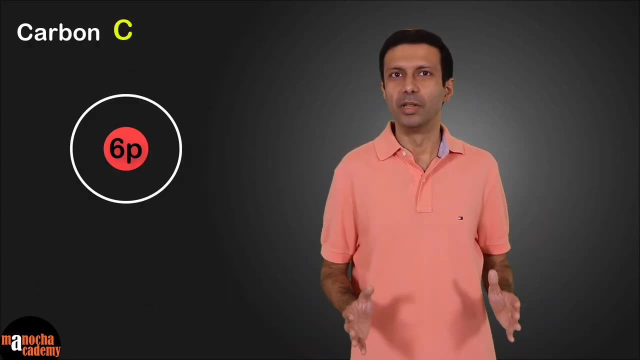 The answer is no. There are certain rules for filling in the electrons in the shells of an atom. These rules are known as Bohr-Berry's rules. So let's go ahead and take a look at these rules. We will start with carbon. 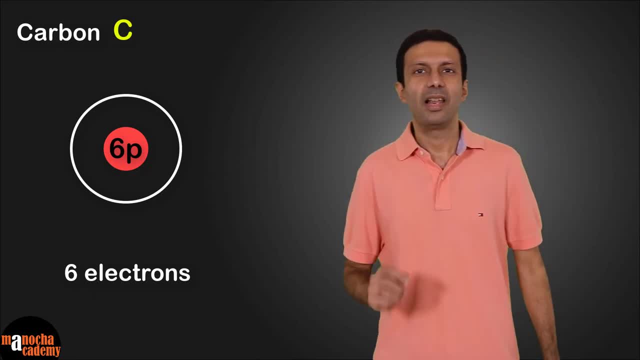 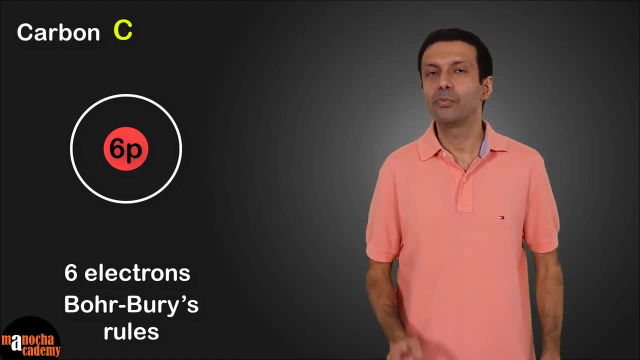 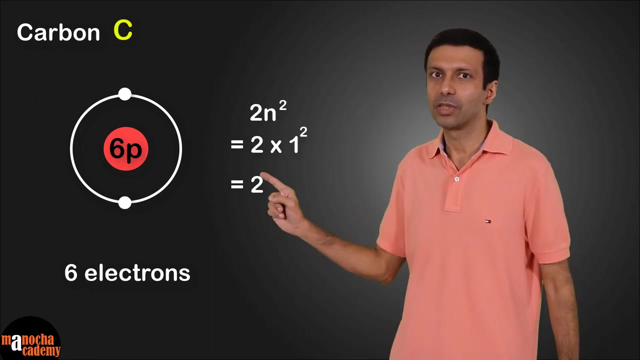 The carbon atom has 6 electrons. Let's fill in the electrons. according to Bohr-Berry's rules, The first shell can hold a maximum of 2n squared, So that's 2 electrons. So let's go ahead and put 2 electrons in the first shell. 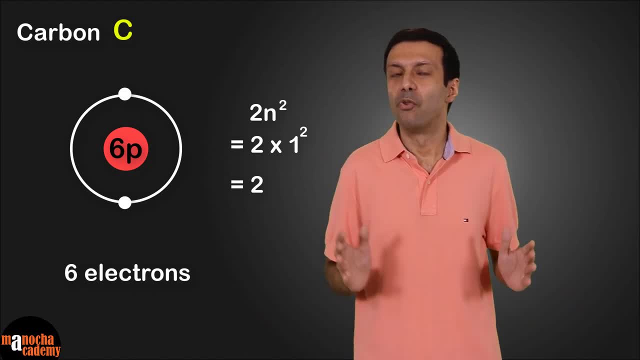 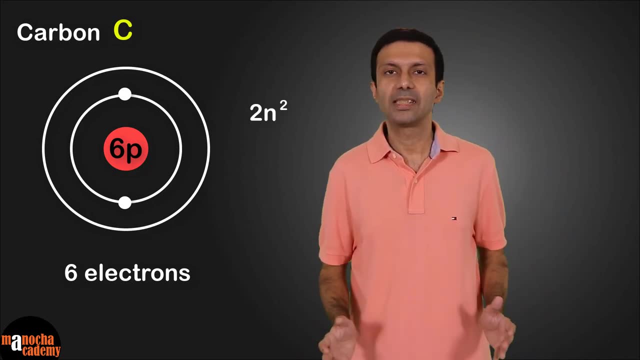 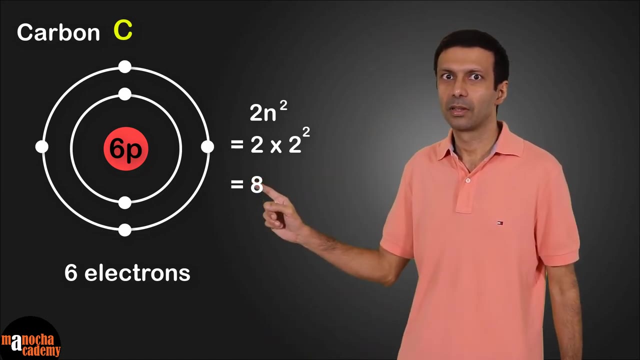 Now how many electrons are we left with? We have 4 electrons. The second shell here can hold a maximum of 2n squared, So that's 8 electrons. So we can put all the 4 electrons in our second shell. The second shell is the outermost shell and it doesn't have more than 8 electrons. 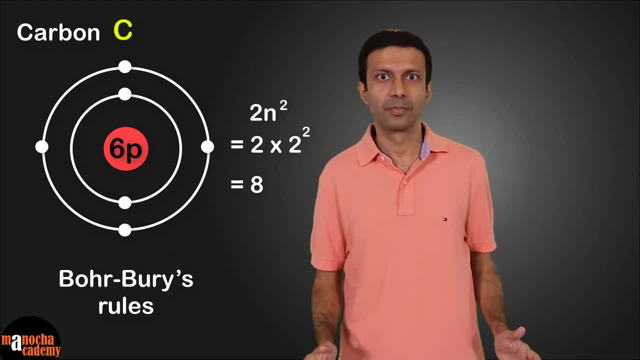 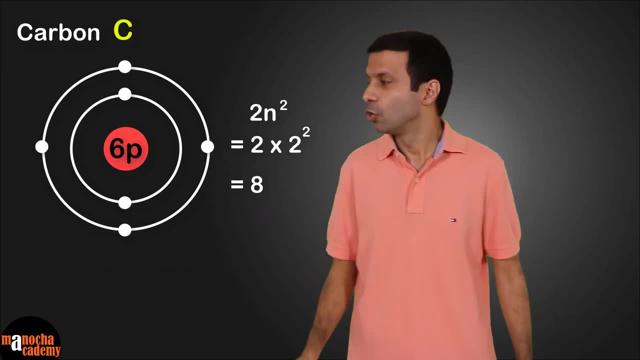 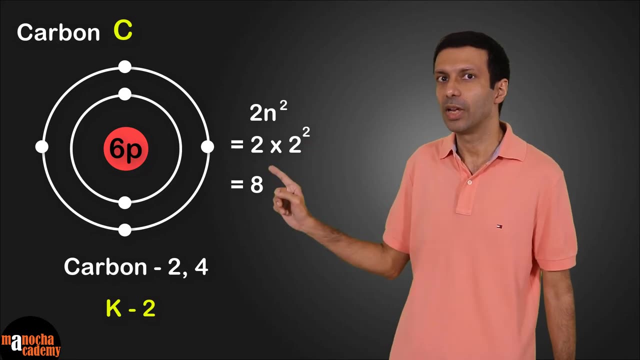 So these shells are following Bohr-Berry's rules And this is the electron configuration diagram of carbon. We can write it in short as 2 comma 4, because the first shell, the k shell, has 2 electrons And the second shell, the l shell, has 4 electrons. 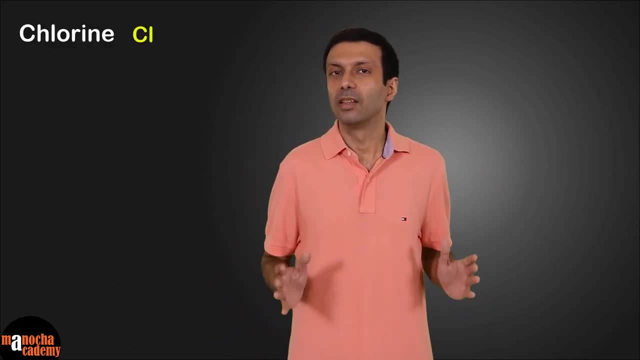 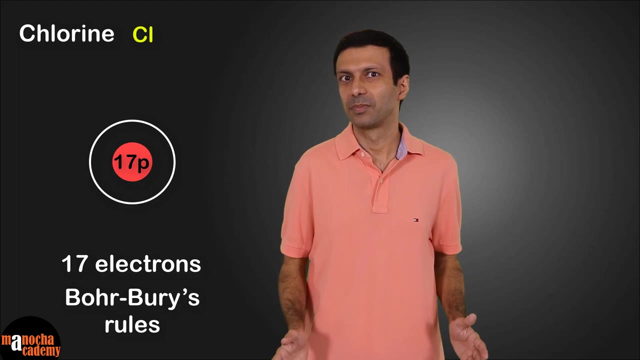 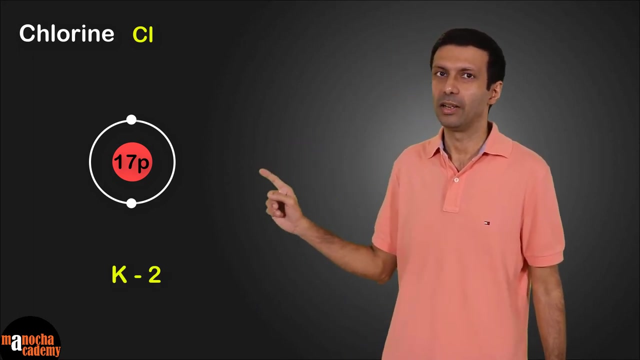 Next let's look at chlorine. The chlorine atom has 17 electrons. Again, we will apply Bohr-Berry's rules. The first shell can hold a maximum of 2 electrons, So let's put in 2 electrons in the first shell. 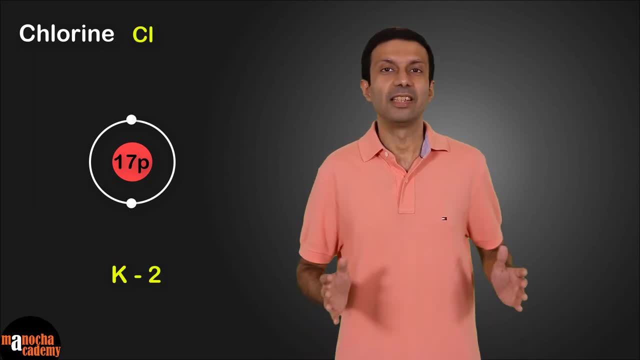 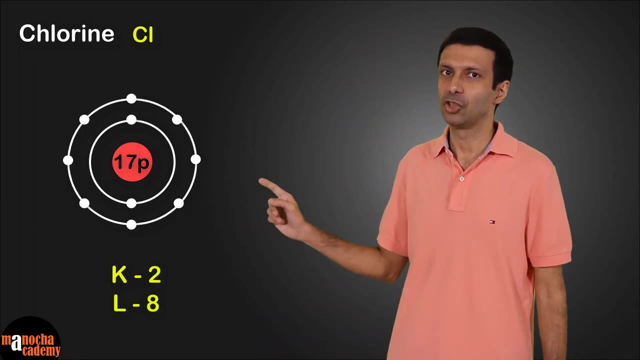 Now we are left with 15 electrons. The second shell can hold a maximum of 8 electrons. So let's fill in 8 electrons in the second shell And we are now left with 7 electrons. The third shell can hold a maximum of 2n squared. 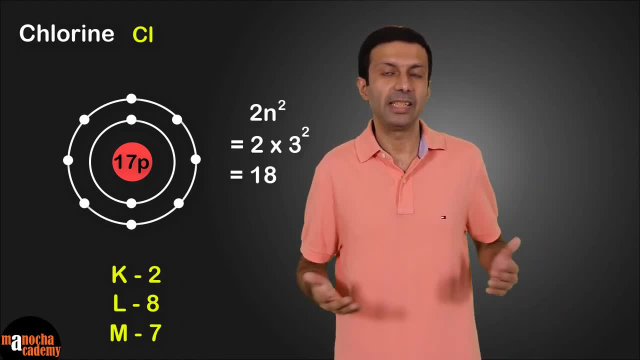 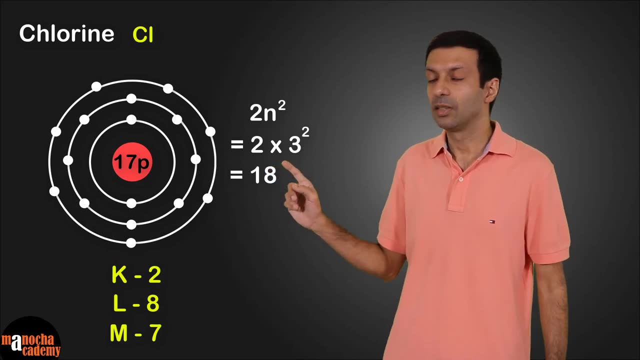 So that's 2 into 3 squared, which is 18 electrons. So we can put in all the remaining 7 electrons in the third shell. The third shell is the outermost shell and it does not have more than 8 electrons. So Bohr-Berry's rules are being followed here. 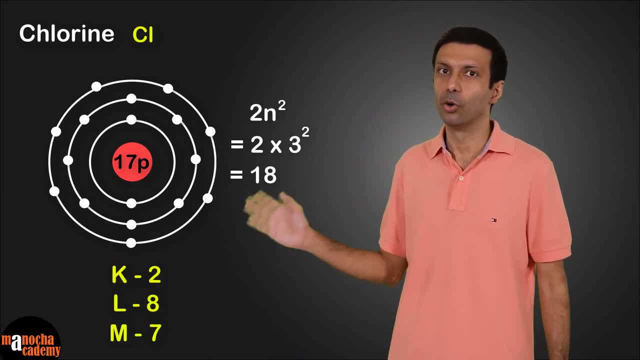 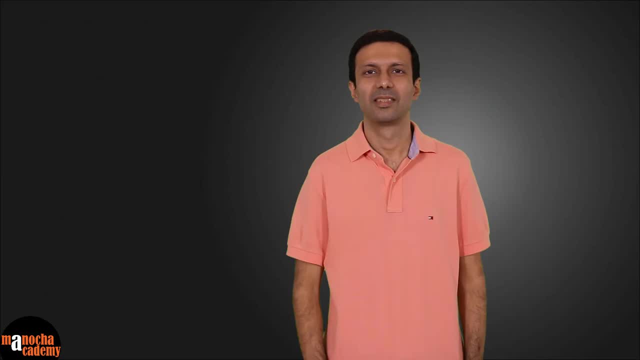 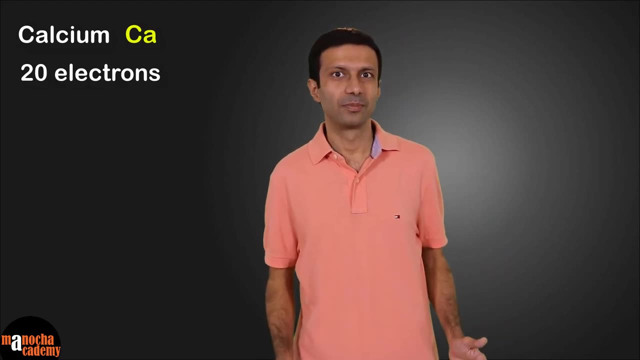 This is our electron configuration diagram of chlorine And, in short, we can write it as 2 comma 8 comma 7.. Next let's try calcium. The calcium atom has 20 electrons This time. why don't you pause the video here and try to get the electron configuration yourself? 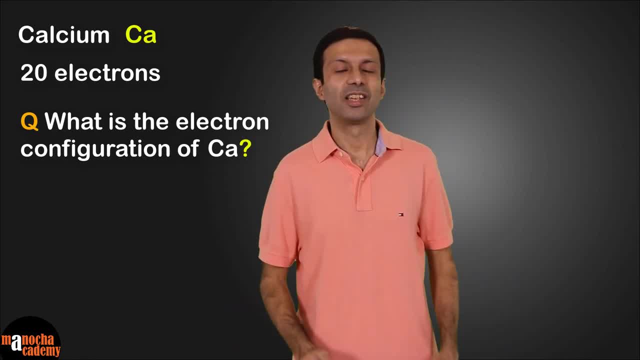 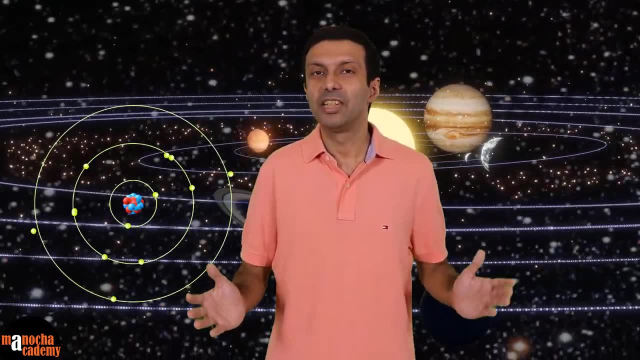 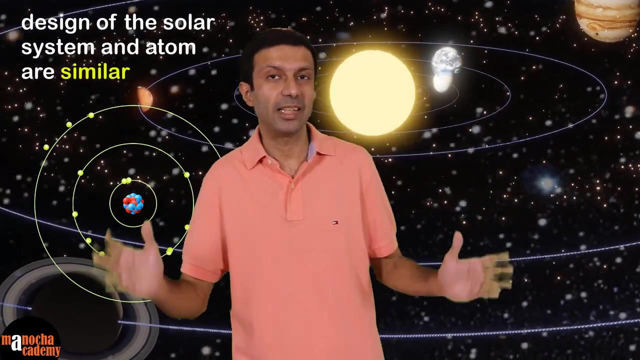 So what did you get? The correct answer is 2 comma 8 comma 8 comma 2.. Isn't it simply amazing that the design of the solar system and the atom are pretty similar? The solar system is this gigantic thing And the atom is a very, very tiny piece.